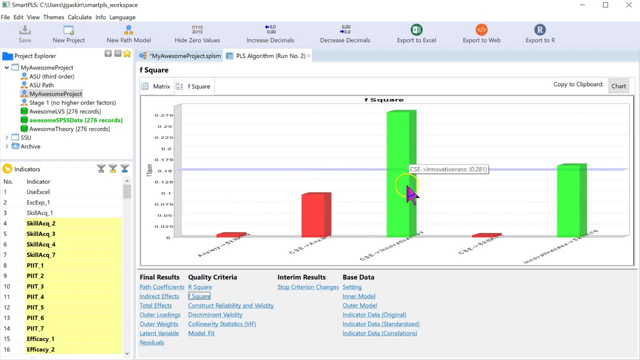 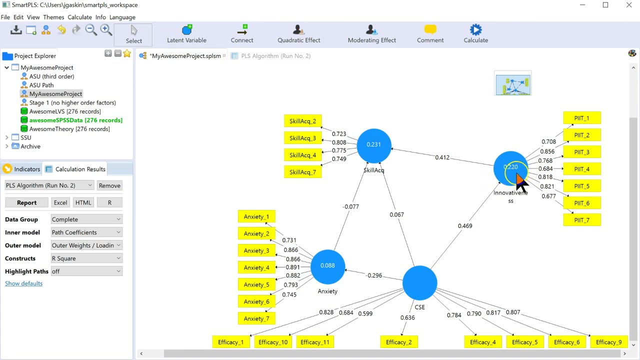 large effect. So we see, here we have only two effects that are considered to be large enough. These are CSE to innovativeness and innovativeness to skill acquisition. Or, if I go look at my model, innovativeness to skill acquisition- Ah yep, that's a fairly large. 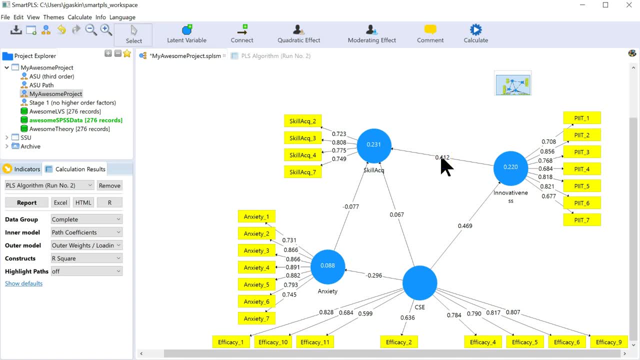 effect. At least the regression weight here is large And if we look at the F-square it shows it's also large. The CSE to innovativeness was our largest effect. Now if we go look at these other values- 0.067, negative 0.077, we can see the regression weight is small And so likely they're not big. 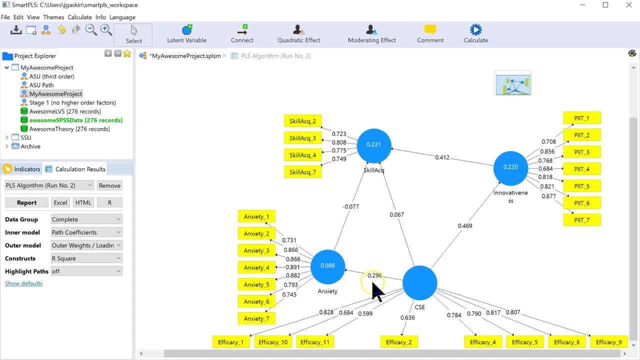 effects And we observed that. But what about this one Negative 0.296.. Seems like a pretty big regression weight And I bet statistically it has a good p-value. Well, to do this, let's go look at the p-values for the coefficient right here. 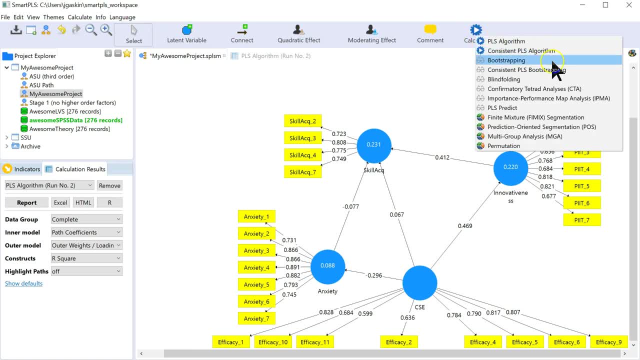 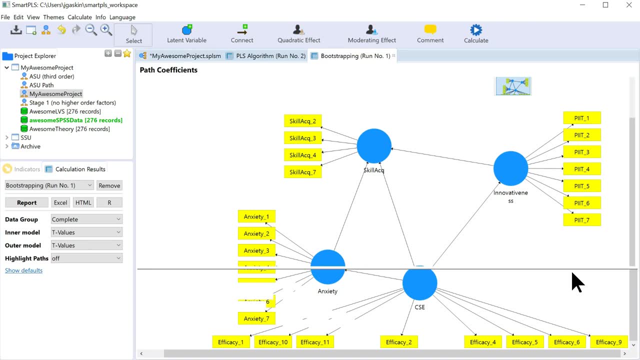 To do that, we need to go to calculate And we're going to do some bootstrapping And I'm just going to accept the defaults: Start report or start calculation. Let it run. Here's the report. And we were looking at what was it? It was CSE to anxiety. 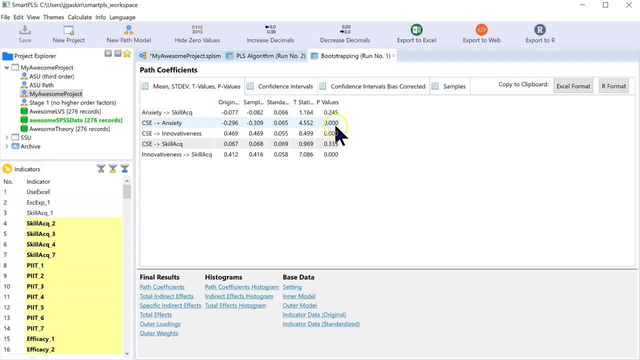 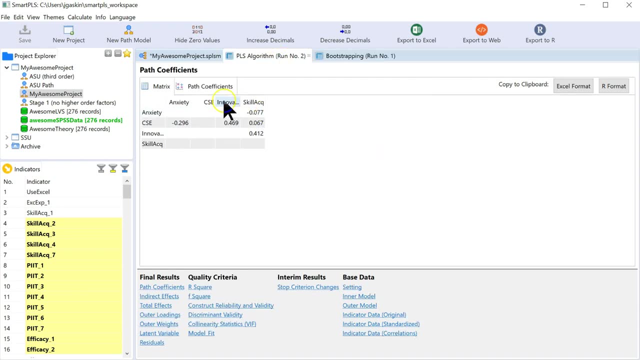 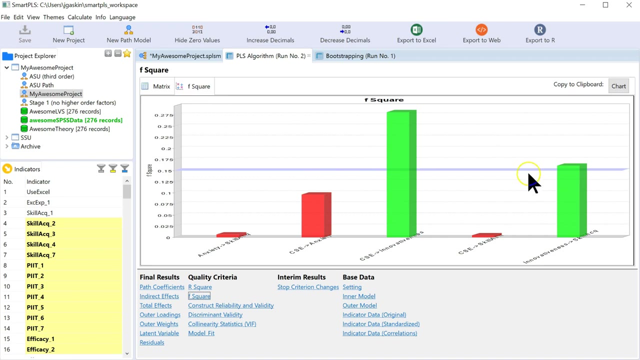 Is it significant? CSE to anxiety Heck, yes, that p-value is so low. It's less than 0.001.. But we learned from our effect sizes right here F square, that even though it is a statistically significant effect, 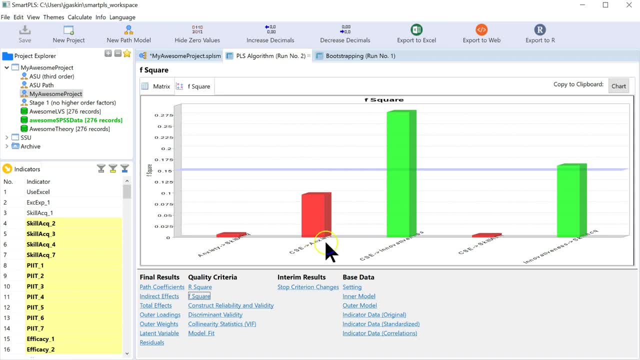 the effect is not meaningful. It is not a big effect. CSE to anxiety. It is less than the 0.15 threshold. In fact it's less than 0.1.. If we were to go and look at the R square not showing now, 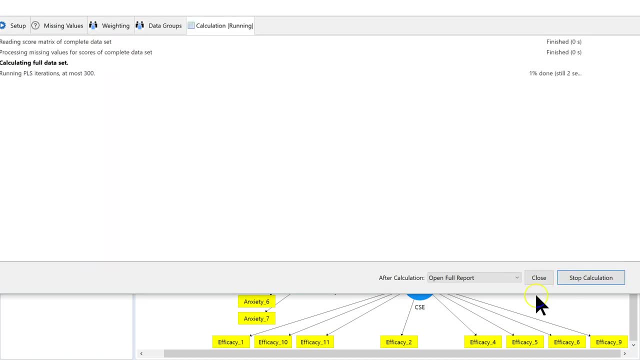 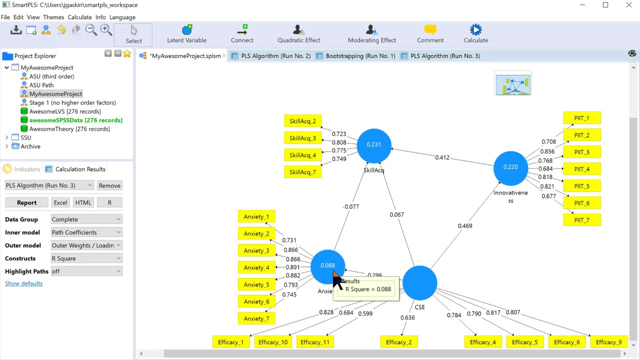 but if I go back and do a PLS algorithm, run it real quick- we'll see that the R square on this is actually very low: 0.088.. So that's a really low R square. So even though we have a 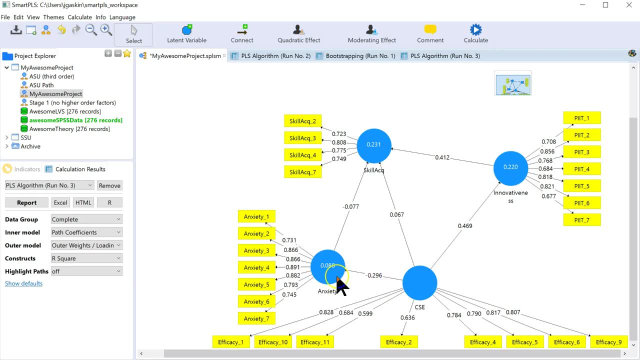 statistically significant coefficient, we're not meaningfully explaining any variance in anxiety, And so that's what you get. by looking at the F square- the effect sizes, You get to see whether your significant effect is actually a meaningful effect. Hope that helps.